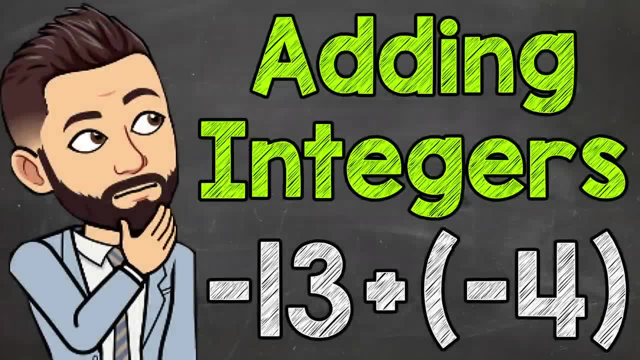 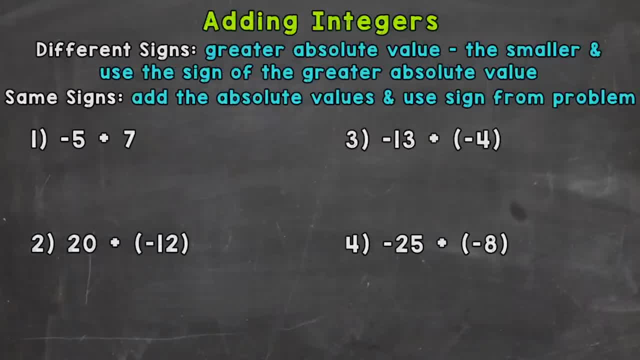 Welcome to Math with Mr J. In this video, I'm going to cover how to add integers. Now, when it comes to adding integers, there are different strategies you can use in order to solve these. So, as we go through the four examples, I'll give you a couple of different ways to think through these problems and get to. 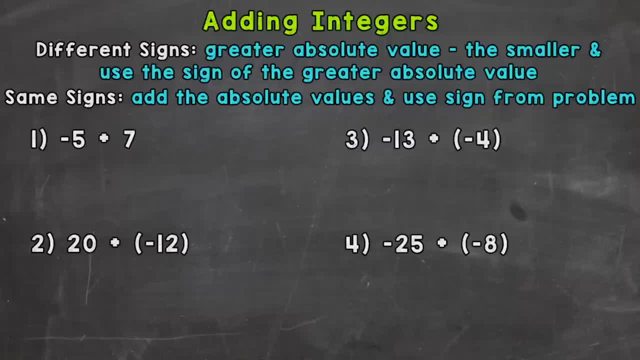 that final answer. So let's jump into number one, where we have negative five plus seven, And the strategy we're going to use first is at the top of the screen. So the first thing we need to do is see if we have different signs or the same signs. In the case of number one, we have 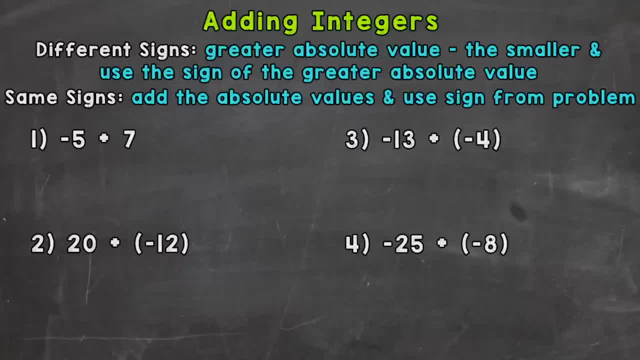 a negative five and a positive seven. So we have different signs, So we're going to look right here. So what we need to do, we need to find the absolute value of our integers And then we'll take the greater absolute value and subtract the smaller absolute value. 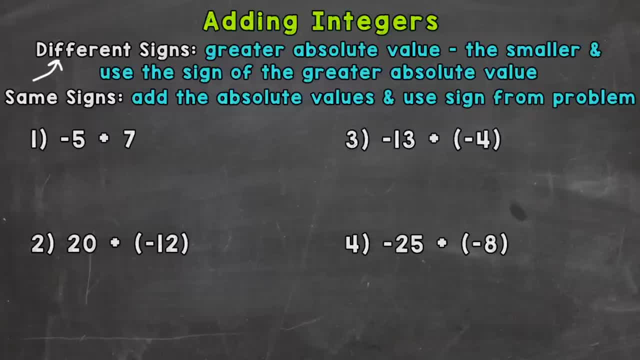 That's going to give us our answer. We'll use the sign of the greater absolute value for that final answer. So let's find our absolute values And remember: absolute value is the distance from zero. The absolute value of negative five is five And the absolute value of seven. 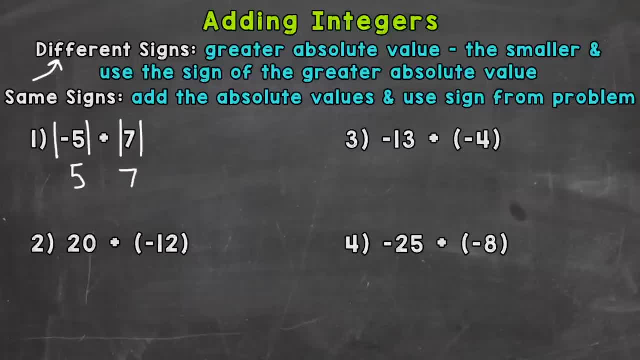 a positive seven is seven. So we take the greater absolute value, which would be seven, and subtract the smaller absolute value, Which is five. Seven minus five is two. Now we need to use the sign of the greater absolute value. So the greater absolute value would be this seven. here And in the original problem. 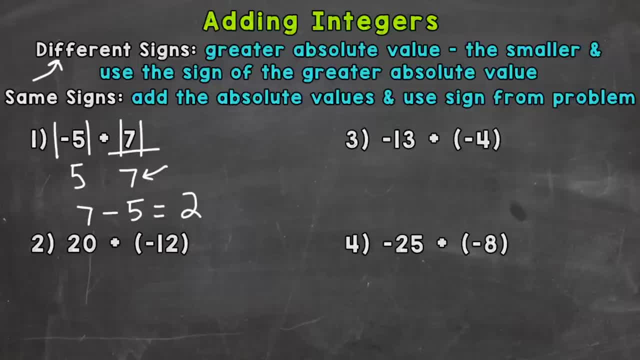 this seven. it's a positive seven, So that means our answer is going to be a positive two. Now the other strategy we can use would be using our overall number sense and knowledge of integers in order to solve this using mental math. So let me rewrite the problem. 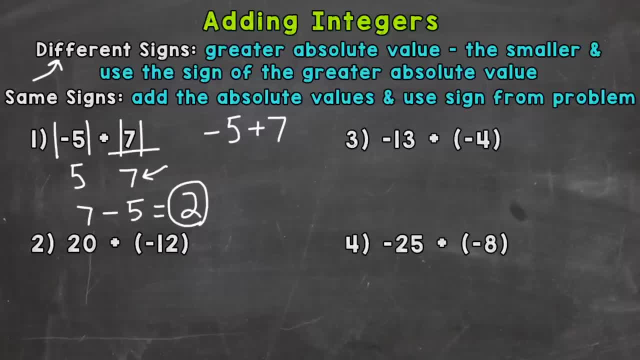 We have negative five plus seven. So one way to think through this problem using mental math would be thinking: okay, we're starting at negative five and we're adding a positive seven, So we are increasing in value. Well, negative five plus a positive five gets us to zero, but we have seven. 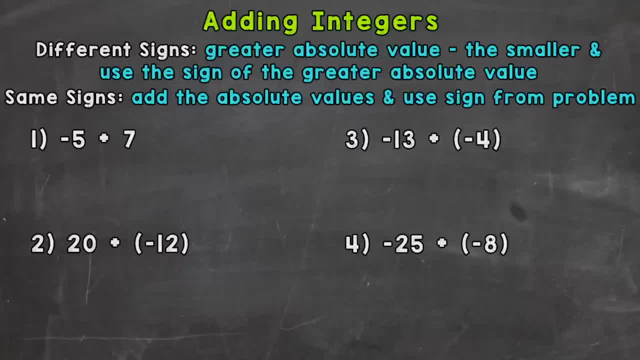 a negative five and a positive seven. So we have different signs, So we're going to look right here. So what we need to do, we need to find the absolute value of our integers And then we'll take the greater absolute value and subtract the smaller absolute value. 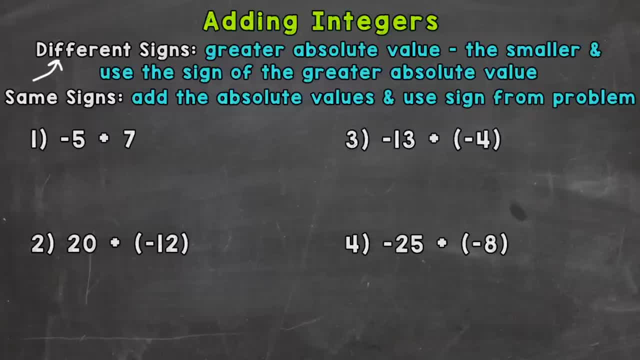 That's going to give us our answer. We'll use the sign of the greater absolute value for that final answer. So let's find our absolute values And remember: absolute value is the distance from zero. The absolute value of negative five is five And the absolute value of seven. 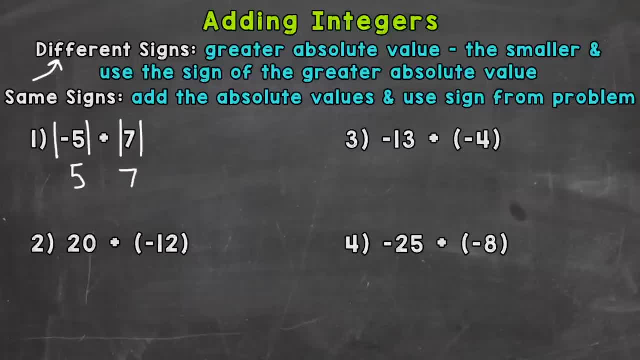 a positive seven is seven. So we take the greater absolute value, which would be seven, and subtract the smaller absolute value, Which is five. Seven minus five is two. Now we need to use the sign of the greater absolute value. So the greater absolute value would be this seven. here And in the original problem. 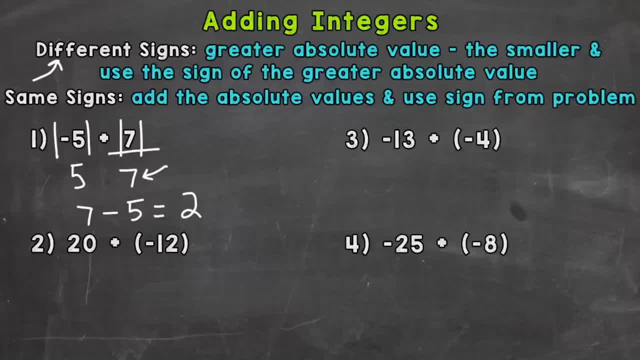 this seven. it's a positive seven, So that means our answer is going to be a positive two. Now the other strategy we can use would be using our overall number sense and knowledge of integers in order to solve this using mental math. So let me rewrite the problem. 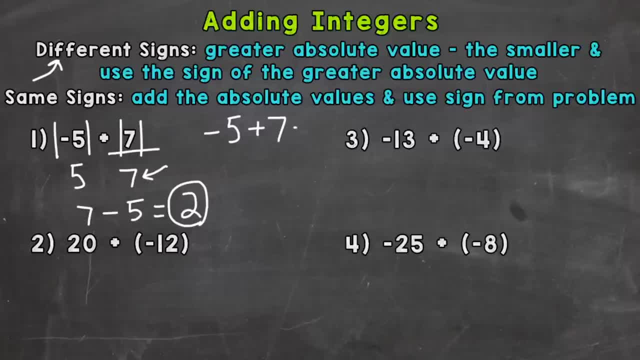 We have negative five plus seven. So one way to think through this problem using mental math would be thinking: okay, we're starting at negative five and we're adding a positive seven, So we are increasing in value. Well, negative five plus a positive five gets us to zero, But we have seven. 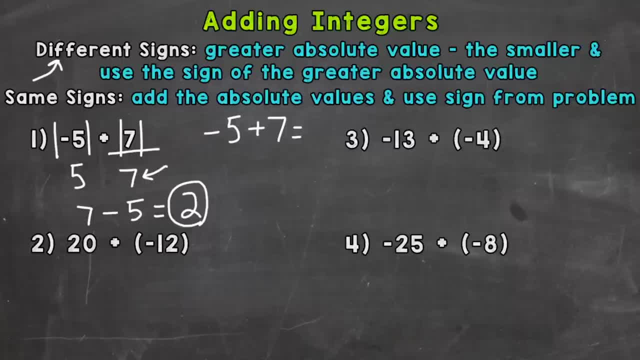 which is two more than that, positive five. So let's go two more than zero And then we're going to add two more than zero And we land on positive two. Now I do want to mention I have a video that goes through how to add integers using a number line, And this really helps visualize what's going on. 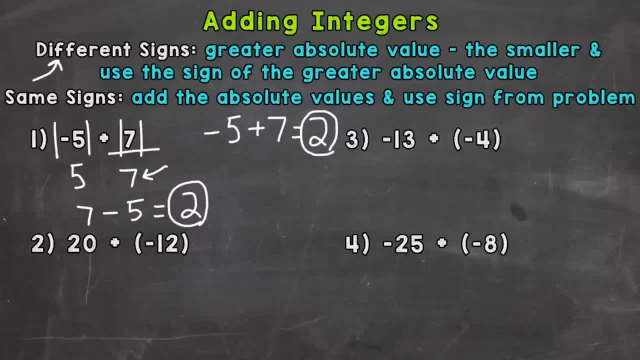 within these problems And it's going to help with mental math. when it comes to adding integers, I'll drop that link down in the description. So let's move on to number two, where we have a positive 20 plus a negative 12.. 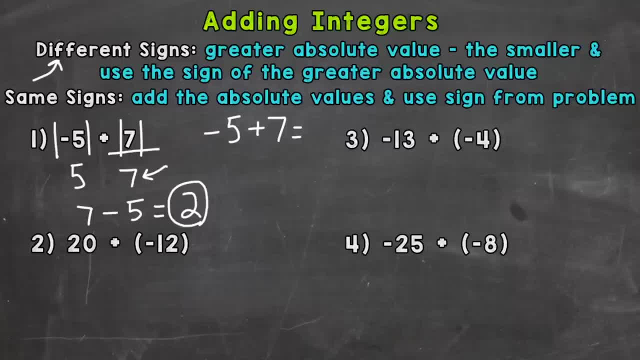 which is two more than that, positive five. So let's go two more than zero And we're going to add two more than zero And we land on positive two. Now I do want to mention I have a video that goes through how to add integers using a number line, And this really helps visualize what's going. 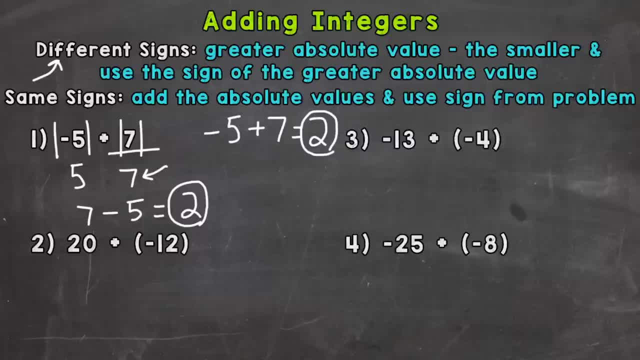 on within these problems And it's going to help with mental math. when it comes to adding integers, I'll drop that link down in the description. So let's move on to number two, where we have a positive 20 plus a negative 12.. 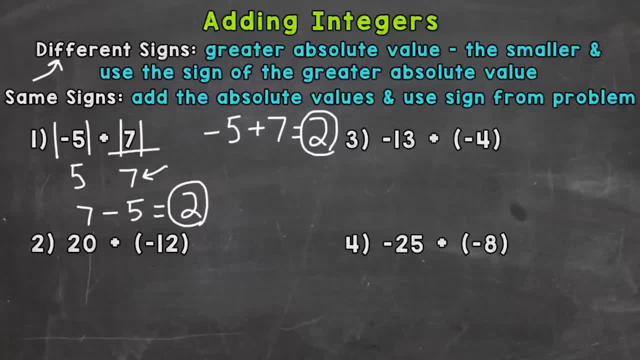 So again we have different signs. So let's find the absolute value of our integers here. So the absolute value of 20 is 20.. And the absolute value of negative 12 is 12.. So we need to do the greater absolute value, 20, minus the smaller absolute value of 12.. And we get eight. So we need to use the sign. 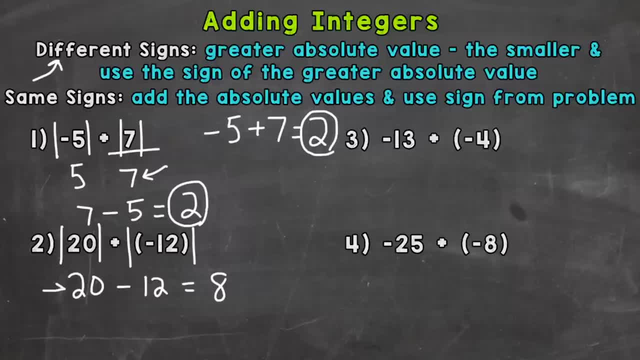 of the greater absolute value, So the greater absolute value of 20 minus the smaller absolute value of 12.. And in the original problem it was a positive 20.. So our answer is a positive eight. Let's think through this using mental math as well. So I'll rewrite the problem: 20 plus negative 12.. So we are. 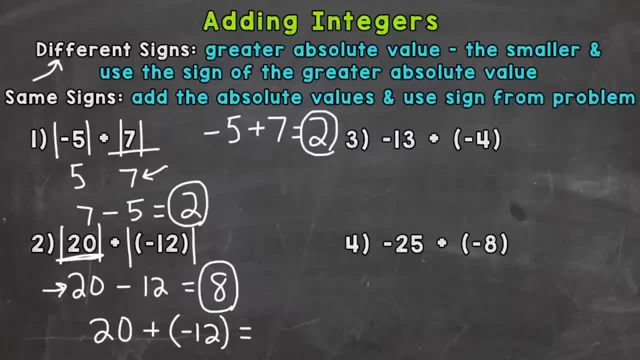 starting at a positive 20.. And we're adding a negative 12.. So we are decreasing in value by 12 from 20.. And we are taking away or subtracting 12 because we are decreasing in value. So we would end up at a. 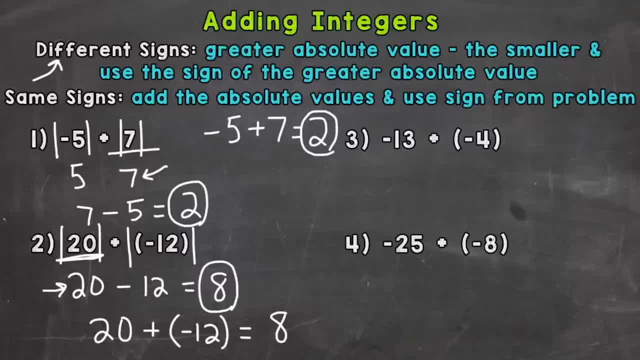 positive eight. Again, we are going from a positive 20. And we are decreasing in value by 12. So we would land on a positive eight for our answer On to number three, where we have negative 13 plus a negative four. 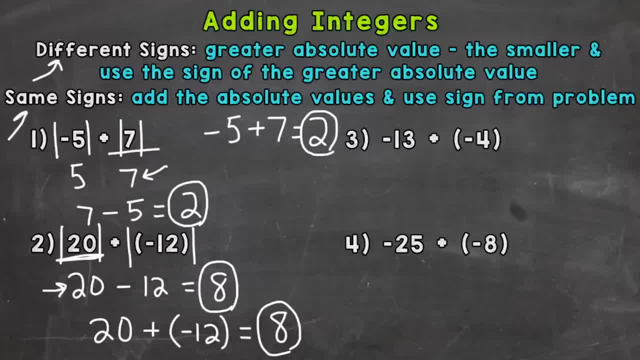 So we have the same signs here. So we will look right here. So we need to add the absolute values and use the same sign from the problem. So let's find our absolute values here. So the absolute value of negative 13 would be 13.. 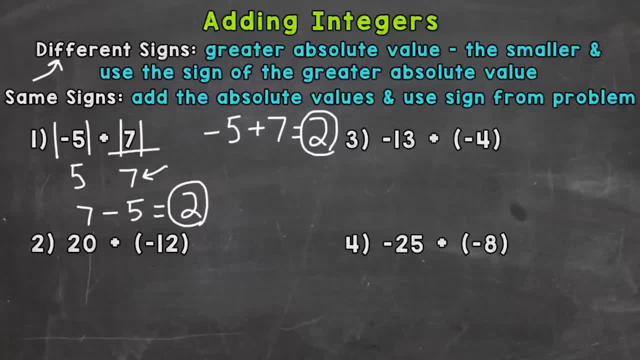 So again we have different signs. So let's find the absolute value of our integers here. So the absolute value of 20 is 20.. And the absolute value of negative 12 is 12.. So we need to do the greater absolute value, 20, minus the smaller absolute value of 12.. And we get eight. So we need to use the sign. 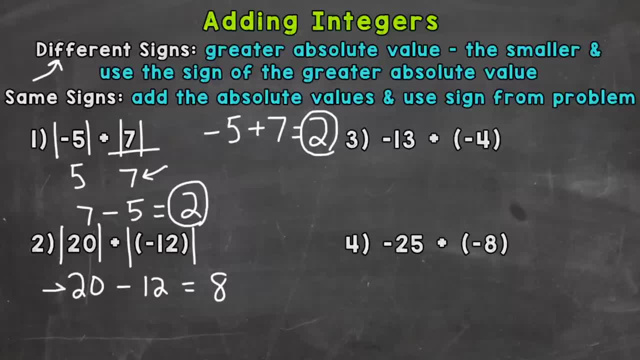 of the greater absolute value. So the greater absolute value of negative 12 is 12.. And we get the negative 20 plus 20 plus negative 12.. And then the first value of the value of negative 12 is 20.. And then the second value of the value of negative 12 is 20.. And in the original problem it was a. 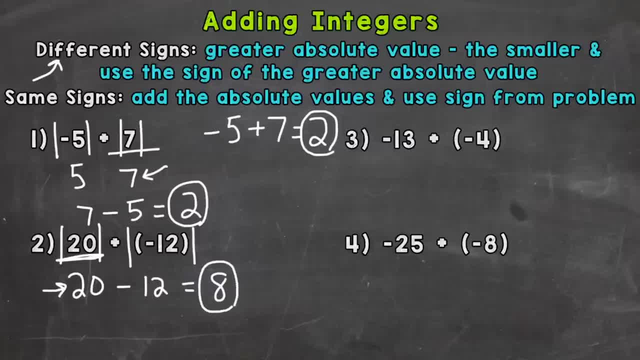 positive 20.. So our answer is a positive eight. Let's think through this using mental math as well. So I'll rewrite the problem: 20 plus negative 12.. So we are starting at a positive 20, and we're adding a negative 12. So we are decreasing in value by 12 from 20.. So we can. 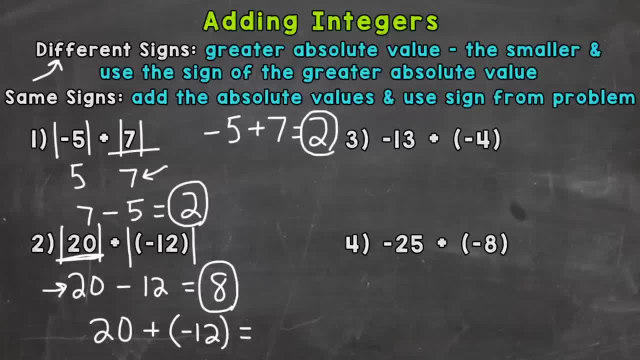 think of this as 20 and we are taking away or subtracting 12 because we are decreasing in value, so we would end up at a positive 8.. Again, we are going from a positive 20 and we are decreasing in value by 12, so we would land on a positive 8 for our answer On to number three, where we have 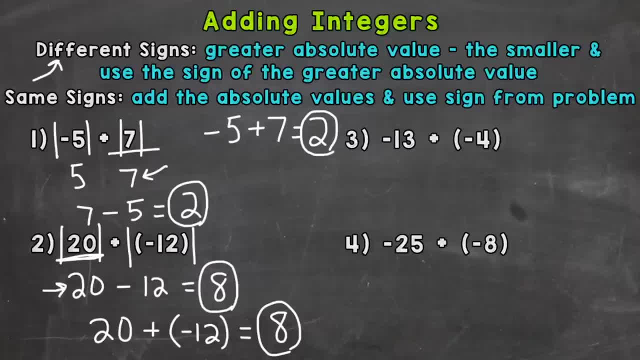 negative 13 plus a negative 4. so we have the same signs here. so we will look right here. So we need to add the absolute values and use the same sign from the problem. So let's find our absolute values here. So the absolute value of negative 13 would be 13. 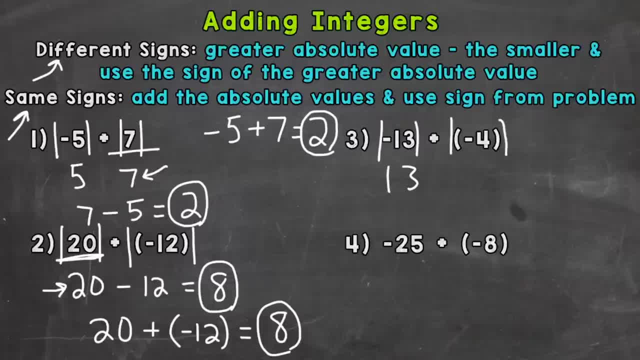 and the absolute value of negative 4 would be 4.. So we need to add the absolute values there. So 13 plus 4 is 17.. And we use the sign from the problem. So the sign from the problem: well, negative 13 and negative 4, both negatives. So our answer is negative 17..